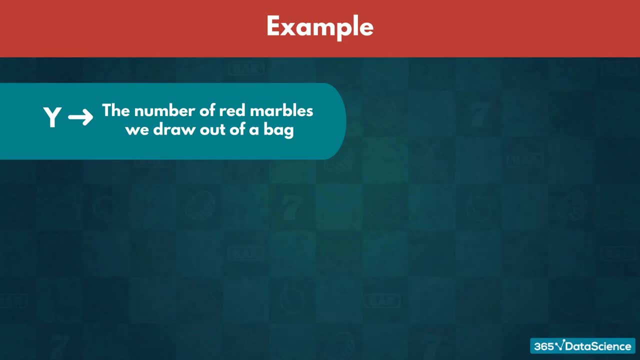 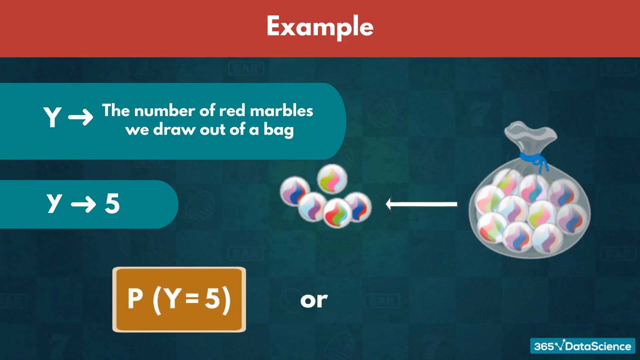 represent the number of red marbles we draw out of a bag And lowercase y would be a specific number like 3 or 5.. Then we express the probability of getting exactly 5 red marbles, as P of Y equals 5 or P of 5.. Since P of Y expresses the probability for 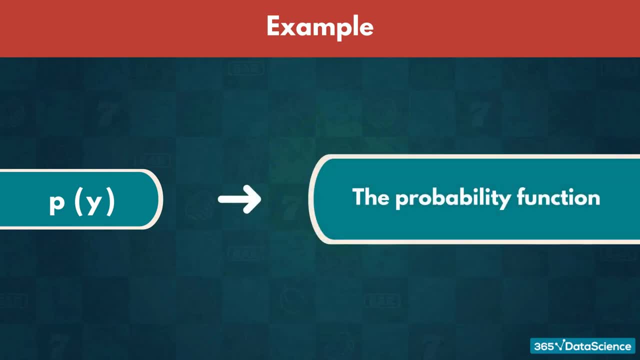 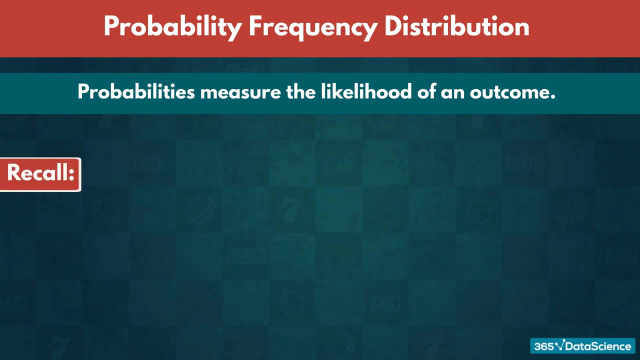 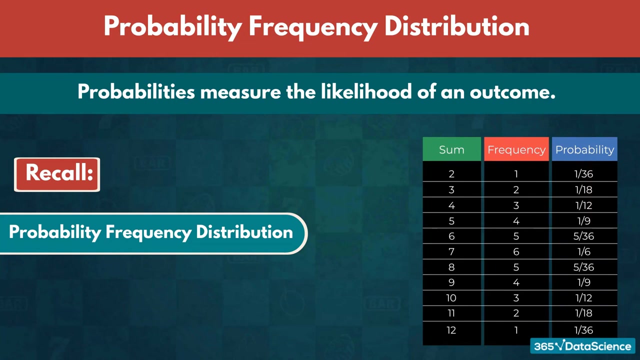 each distinct outcome. we call this the probability function. Good job folks. So probability distributions, or simply probabilities, measure the likelihood of an outcome depending on how often it is featured in the sample space. Recall that we constructed the probability frequency distribution of an event in the introductory section of the course. 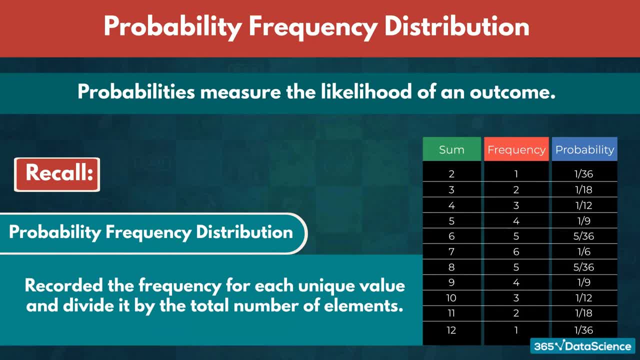 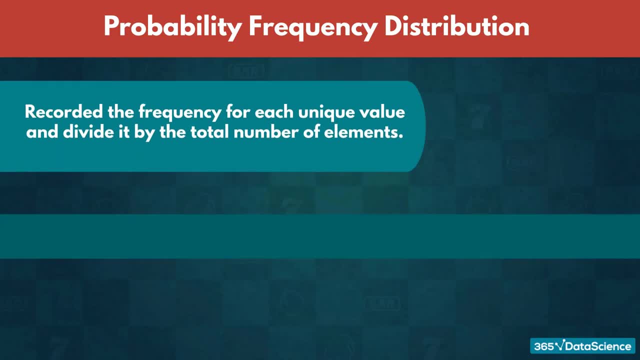 We recorded the frequency for each unique value and divided it by the total number of elements in the sample space. Usually that is the way we construct these probabilities when we have a finite number of possible outcomes. If we had an infinite number of possibilities, then recording the frequency for each one becomes impossible. 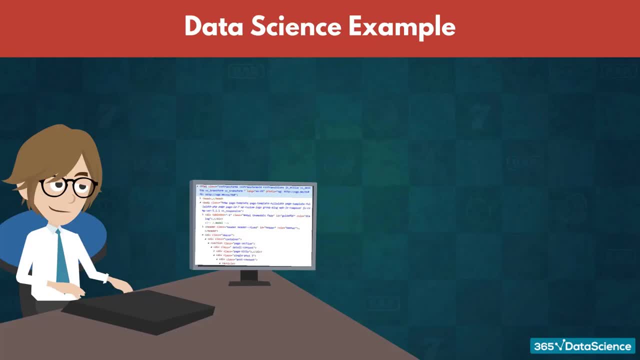 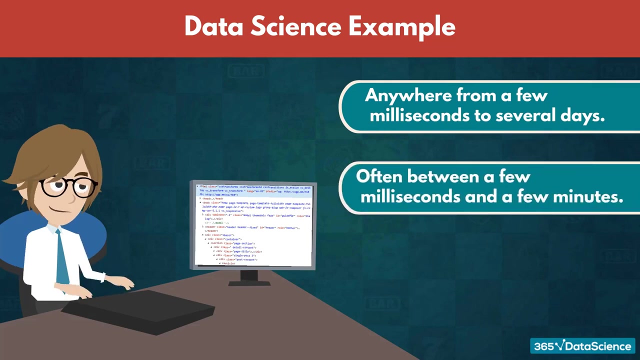 because there are infinitely many of them. For instance, imagine you are a data scientist and want to analyze the time it takes for your code to run. Any single compilation could take anywhere from a few milliseconds to several days. Often, the result will be between a 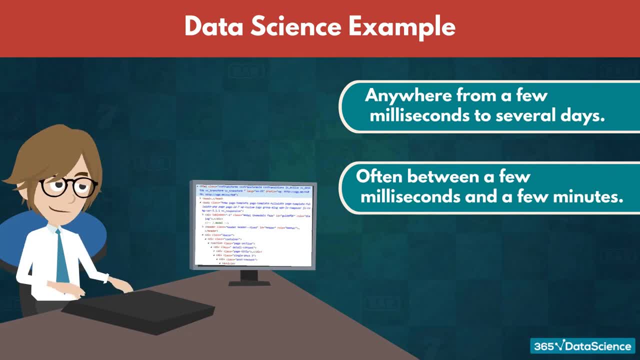 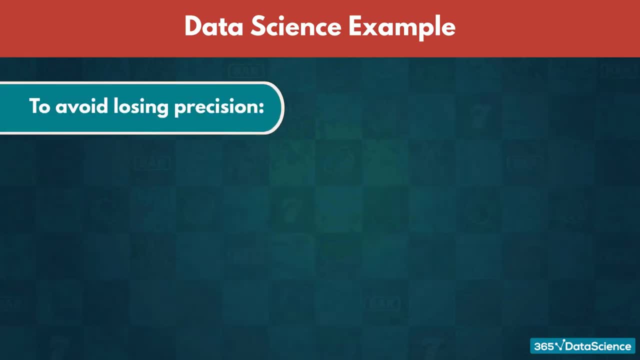 few milliseconds and a few minutes. If we record time in seconds, we lose precision, which is something to be avoided. To do so, we need to use the smallest possible measurement of time, Since every milli, micro or even nanosecond could be split in half. 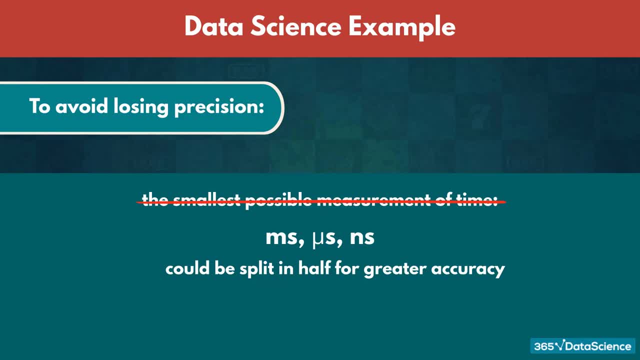 for greater accuracy. no such thing exists. In less than an hour from now, we will talk in more detail about continuous distributions and how to deal with them. Now is the time to introduce some key definitions, Regardless of whether we have a finite or 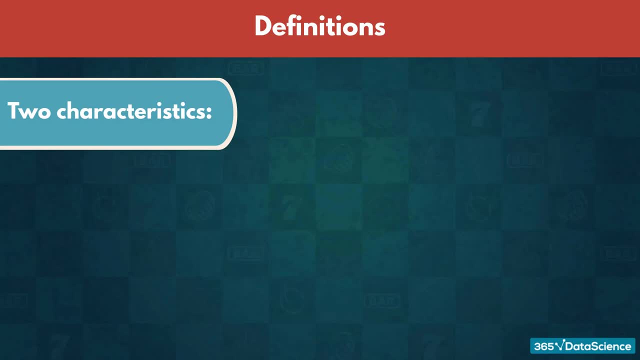 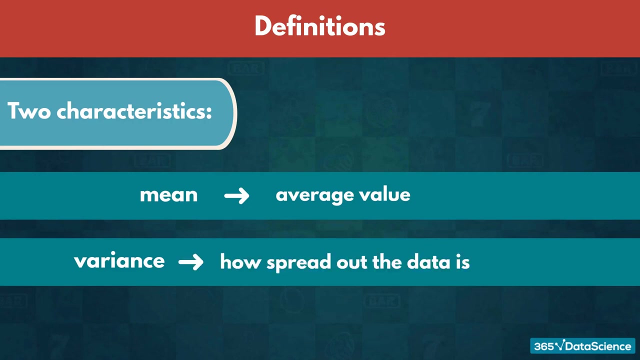 infinite number of possibilities. we define distributions using only two characteristics – mean and variance. Simply put, the mean of the distribution is its average value. Variance, on the other hand, is essentially how spread out the data is. We measure this spread by how far away from the mean all the values are, The more dispersed the data is. 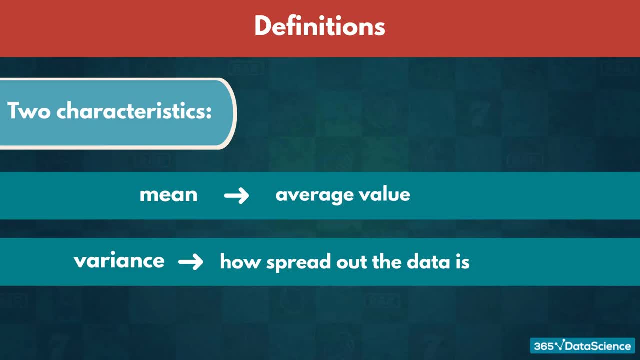 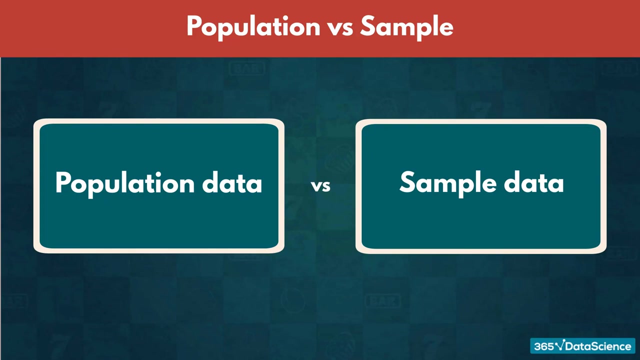 the higher its variance will be. We denote the mean of a distribution with the Greek letter mu and its variance with sigma squared Ok. when analyzing distributions, it is important to understand what kind of data we are dealing with – population or sample data? Population data is the formal way of referring to all. 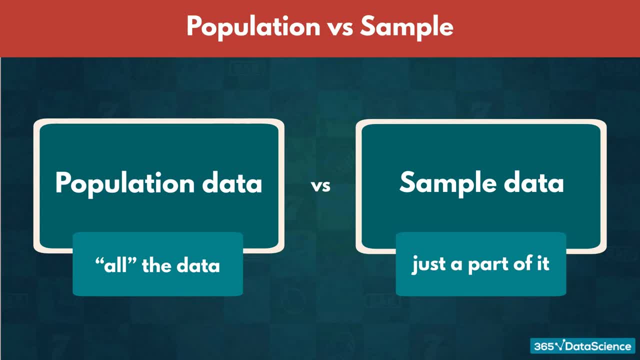 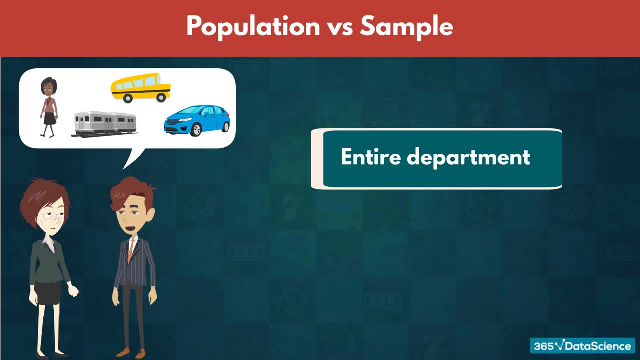 the data, while sample data is just a part of it. For example, if an employer surveys an entire department about how they travel to work, the data would represent the population of the department. However, this same data would also just be a sample of the employees. 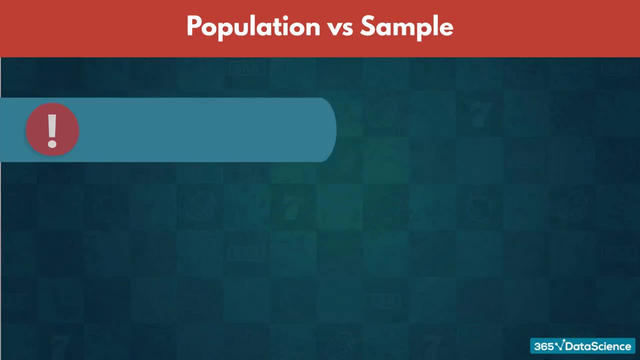 in the whole company. Something to remember when using sample data is that we adopt different notations for the mean and variance. We denote sample mean as x-bar and sample variance as s-squared. One flaw of variance is that the variance is not the same as the sample variance. The variance 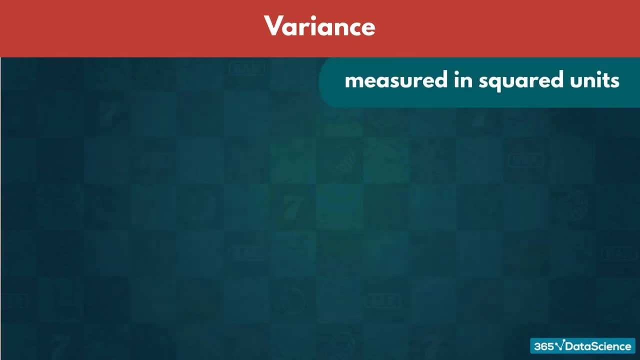 is that it is measured in squared units. For example, if you are measuring time in seconds, the variance would be measured in seconds squared. Usually there is no direct interpretation of that value. To make further sense of variance, we introduce a third characteristic of the distribution. 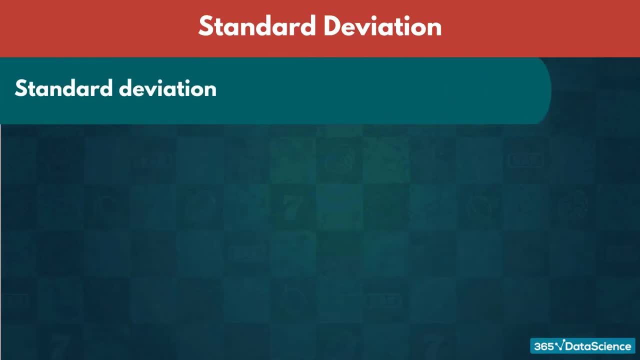 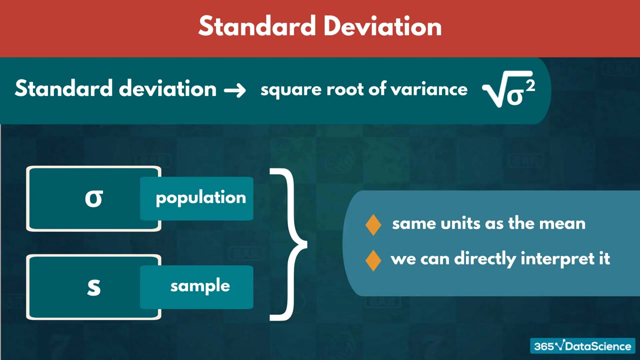 called standard deviation. Standard deviation is simply the positive square root of variance. As you may suspect, we denote it as sigma when dealing with a population And as s when dealing with a sample. Unlike variance, standard deviation is measured in the same units as the mean. Thus we can directly interpret it and is often preferable. 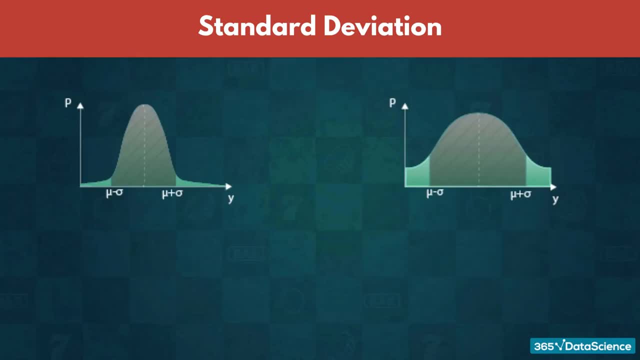 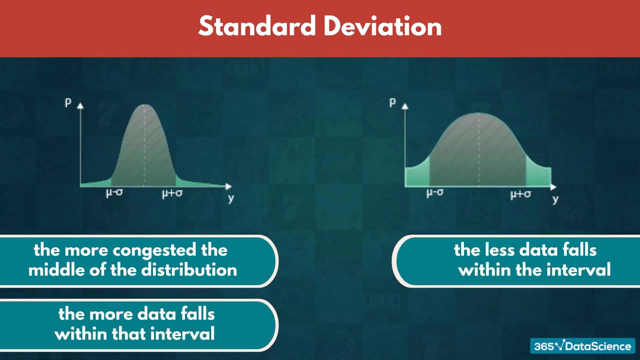 One idea which we will use a lot is that any value between mu minus sigma and mu plus sigma falls within one standard deviation away from the mean. The more congested the middle of the distribution, the more data falls within that interval. Similarly, the less data that falls within the interval, the more dispersed the data. 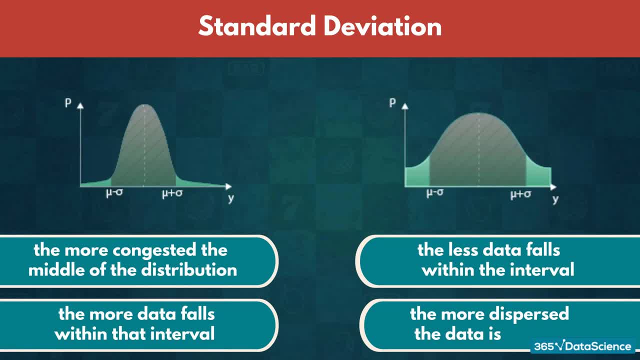 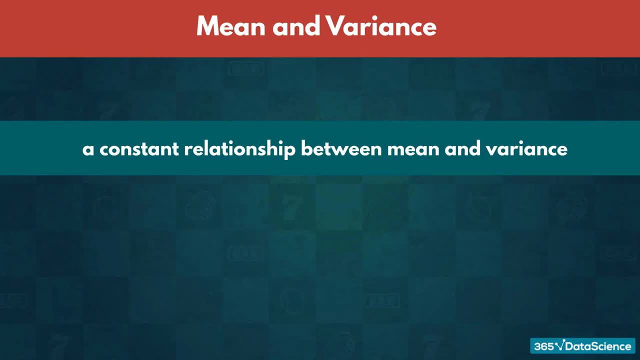 is Fantastic. It is important to know that a constant relationship exists between mean and variance for any distribution. By definition, the variance equals the expected value of the squared difference from the mean for any value. We denote this as sigma squared equals the expected value of y minus mu squared.